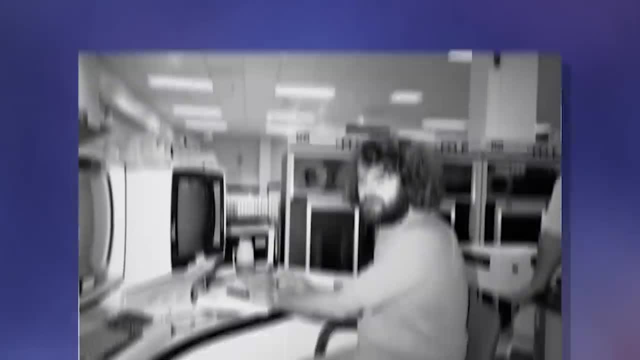 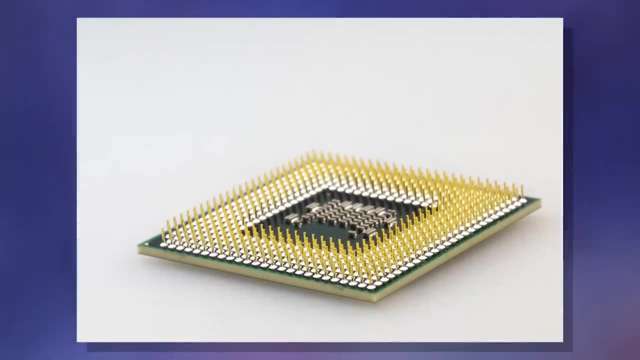 using an assembler that translates the human readable code into 1s and 0s. Assembly is one of the world's first programming languages. It used to be the standard to run supercomputers back in the day, but you still find it used currently to work with CPU memory and it's 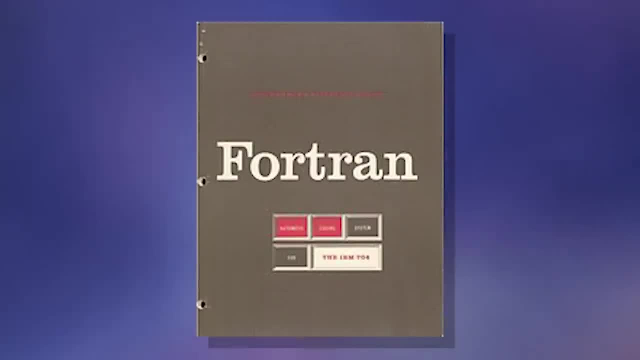 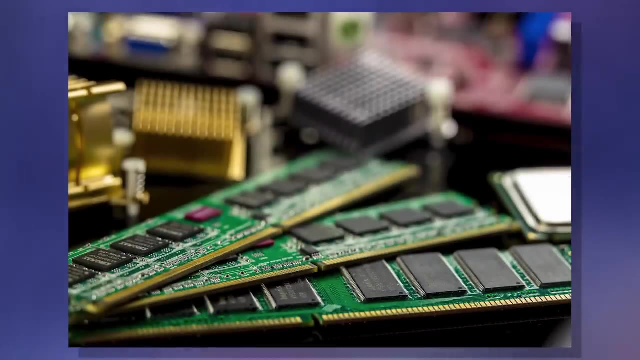 used sometimes in browsers via WebAssembly Fortran, one of the world's first high-level languages. The difference between a high-level language and a low-level language is: in a low-level language you can manipulate the computer's memory much more directly. It also 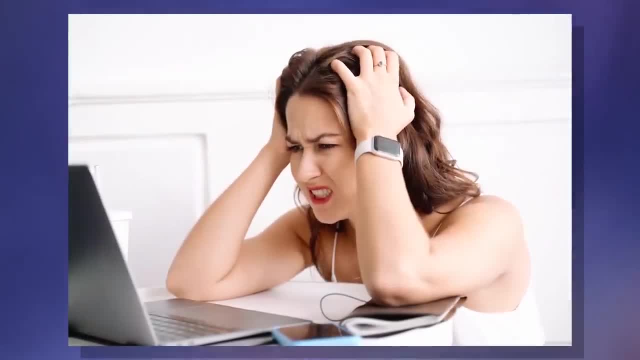 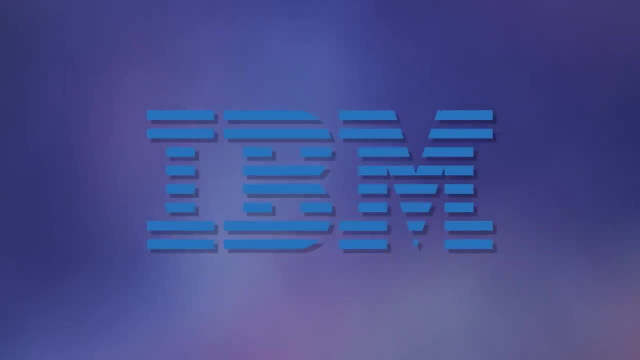 executes much faster than a high-level language. The drawback is that it's much harder to learn. A high-level language is much easier to understand and there's a lot of support, but the code is much slower. Fortran was created by IBM in the 1950s. The name stands for a formula. 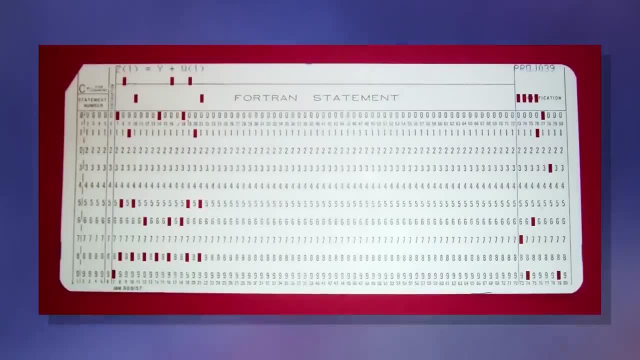 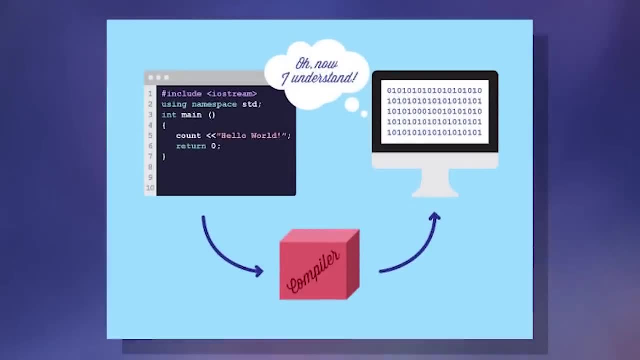 translator. Programming in Fortran would be done by using a punch card, then would be fed into a card reader and would be translated into code that the computer can understand. This translating process is called compiling, which basically changes the code that humans can read into the ones and zeros. 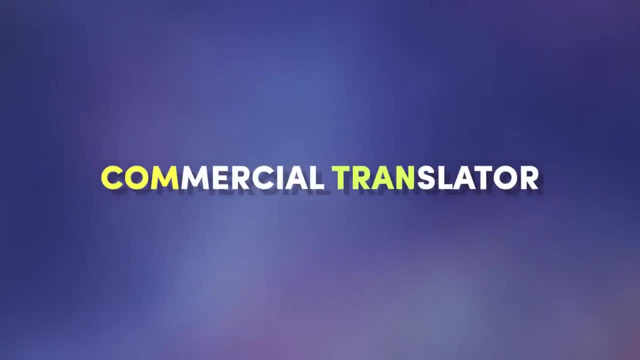 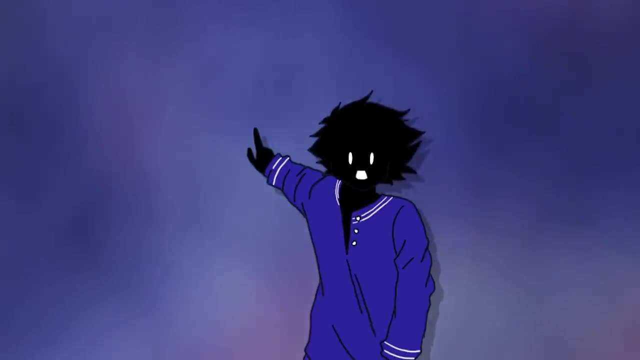 computers can understand. Comtran, also known as commercial translator, is another programming language developed by IBM. It served as the business equivalent to Fortran, in which Fortran was used for scientific computing. It was influenced by another programming language called Flomatic. 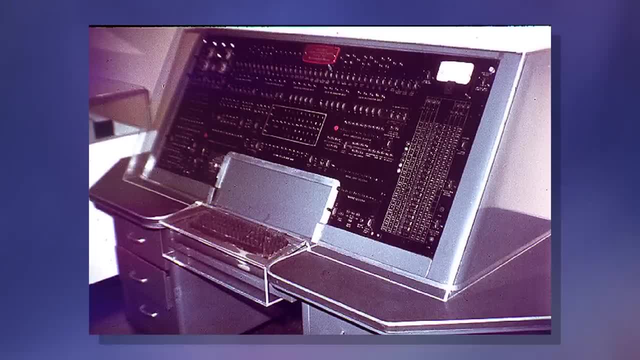 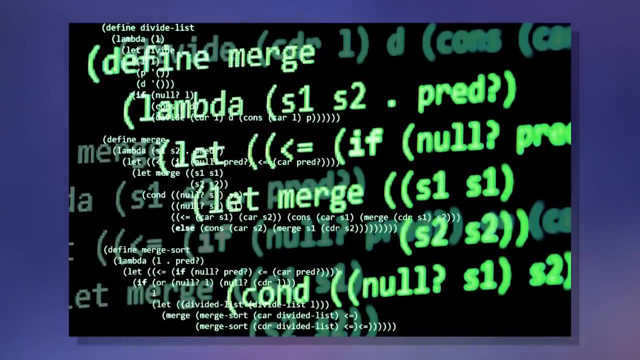 a programming language for data processing that ran on this giant supercomputer called the UNIVAC-1.. Lisp, also known as list processing, was created soon after Fortran. It's known for using a lot of parentheses in its code. The code is also used for programming languages, which inspired these concepts in programming. 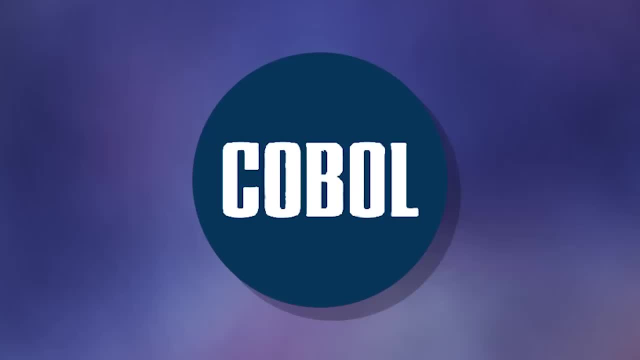 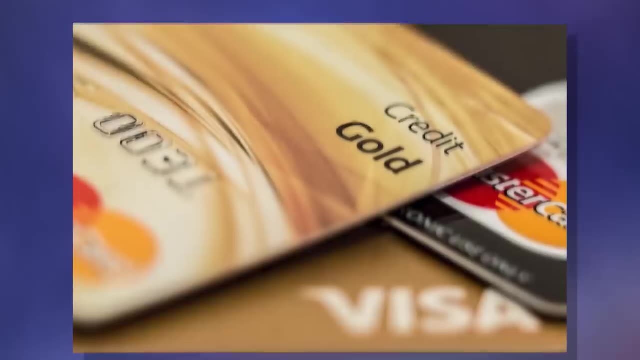 COBOL, standing for Common Business Oriented Language, was the programming language developed in 1959 for- you guessed it- businesses. Even though it was made so long ago, it is still used today by many financial institutions to process transactions. The code looks like: 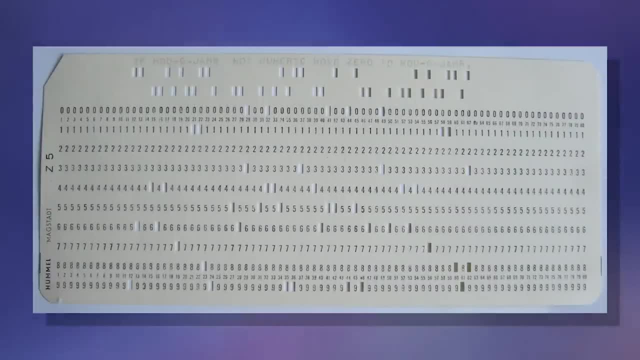 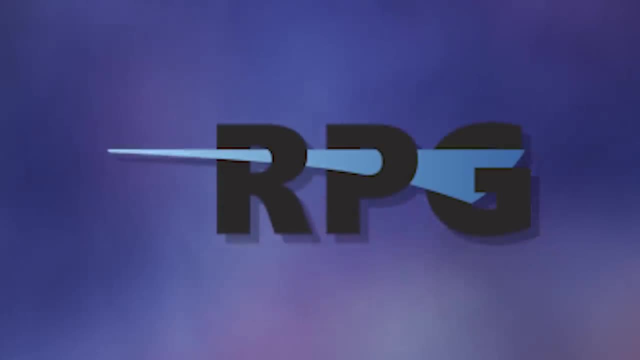 plain English sentences, but this would later be translated onto a punch card. One of the first adopters of the language was the US Department of Defense. IBM RPG- IBM Report Program Generator is a programming language created by IBM meant to run on IBM. 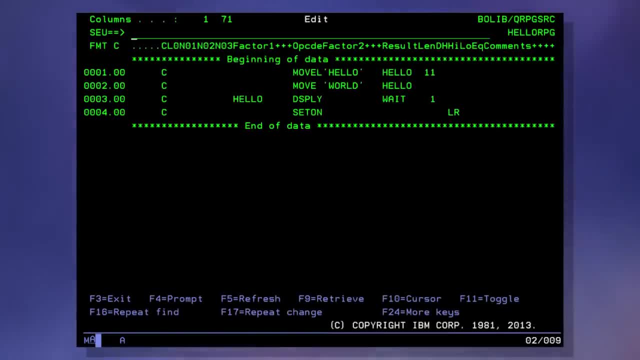 systems. It's one of the only programs that can be used by IBM to run on IBM systems. It is the only programming language to make use of rows and columns for its code, ALGOL-60, short for Algorithmic Language 1960, is not a very well-known programming language. 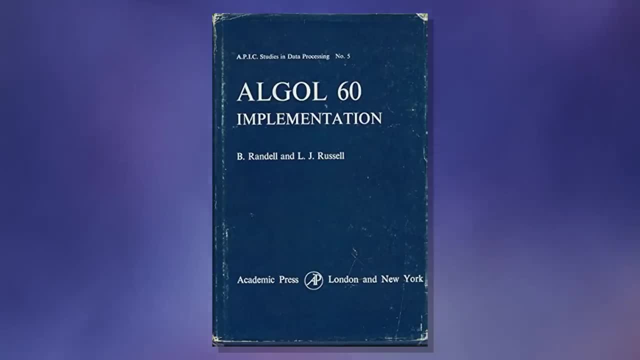 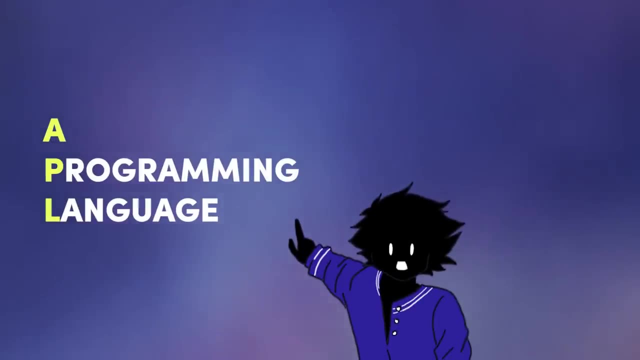 but is one of the languages that inspired one of the most well-known programming languages in the world- C. It was also one of the first programming languages to use nested functions. APL- standing for A Programming Language- first appeared in the 1960s. is a programming. 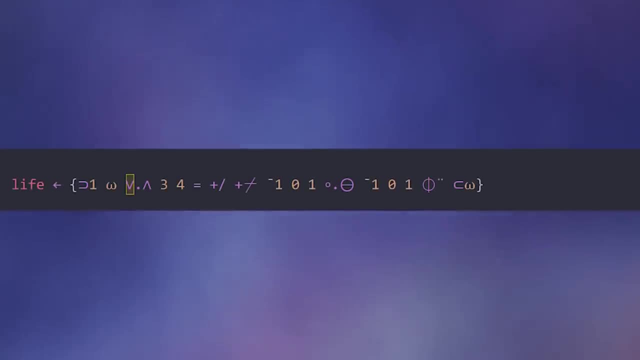 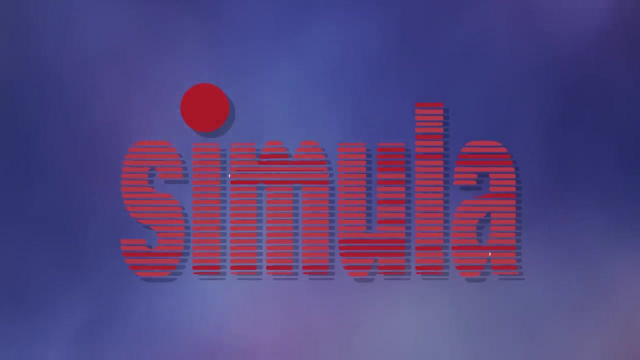 language developed for mathematical equations, mostly algebra. It uses a lot of math and Greek symbols directly in the code SIMULA. In fact, many decades ago that was one of the world's first object-oriented language. Object-oriented programming is a way for programmers to use blocks of code that are reusable and 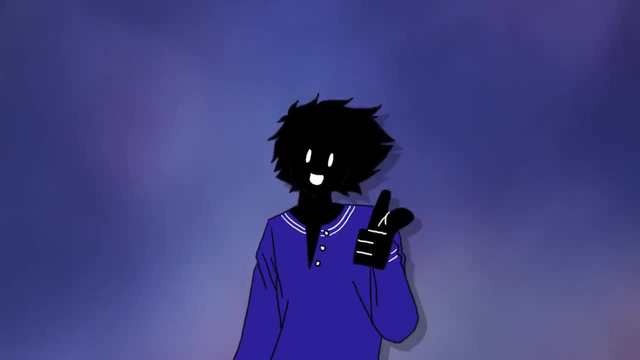 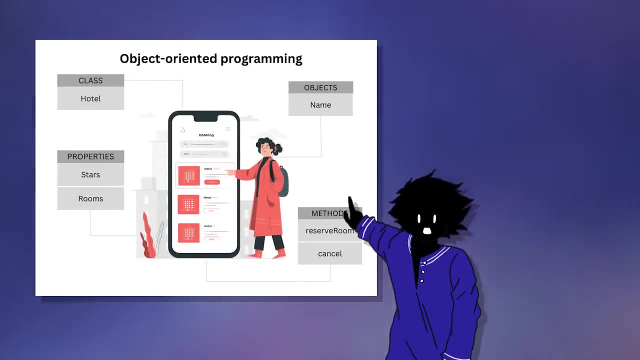 can interact with each other. instead of pure functions and logic. In object-oriented programming, you use blocks of code called objects. Objects are created by things called classes, which contain properties and can use methods. To explain it simply, you can create a class called Pokemon, name the object Charmander. 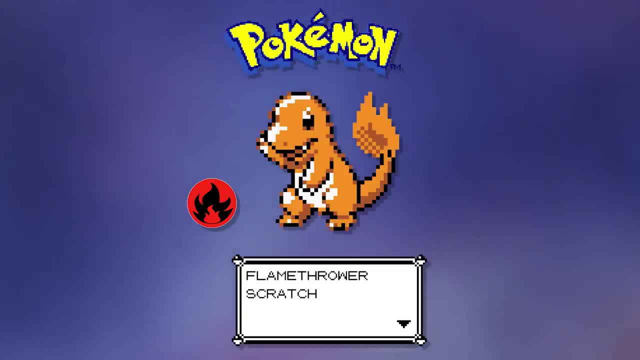 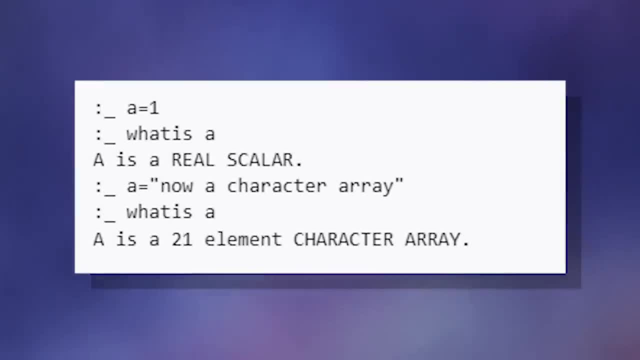 give it properties such as FireType and allow it to execute methods such as Flamethrower and Scratch. APL is a programming language that was mainly used by physicists in the 60s. It's known for using a colon underscore in its code. 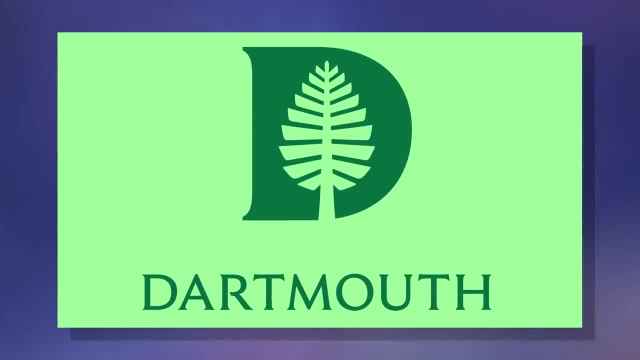 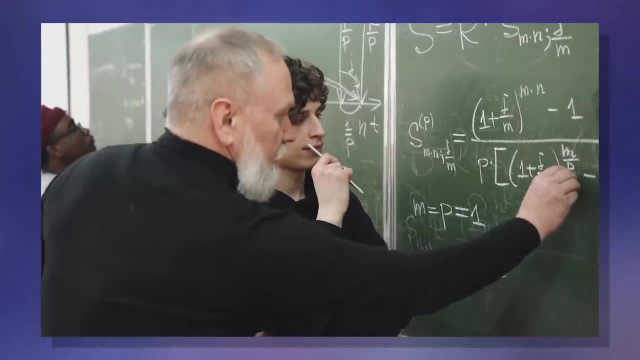 BASIC, The Beginner's All-Purpose Symbolic Instruction Code, was created at Dartmouth in 1963. It was created with the purpose of getting the average layperson to be able to learn how to code. You see, before that time, programming had only been the domain of scientists and mathematicians. 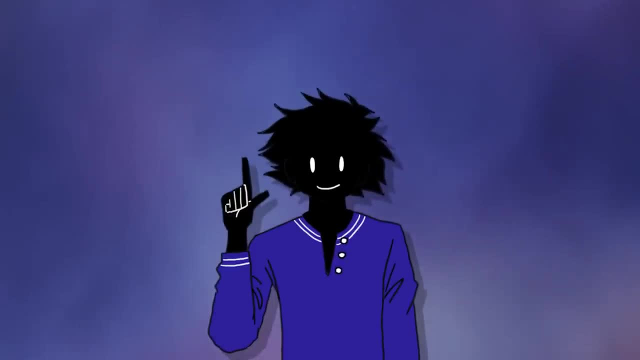 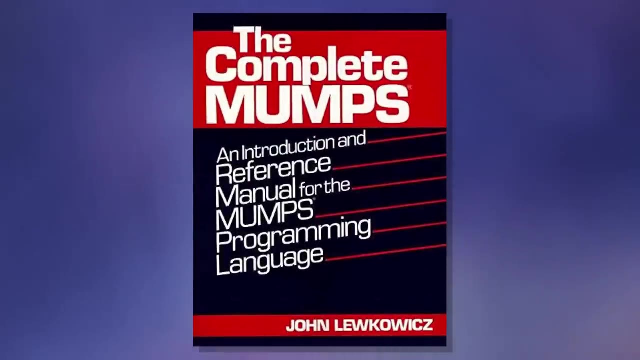 This was because of its easy-to-understand syntax. Syntax is basically the rules to writing in a programming language. MUMPS- MUMPS, aka the Massachusetts General Hospital Utility Multi-Programming System, or MUMPS, or sometimes just M for short, was created to manage hospital laboratory information. 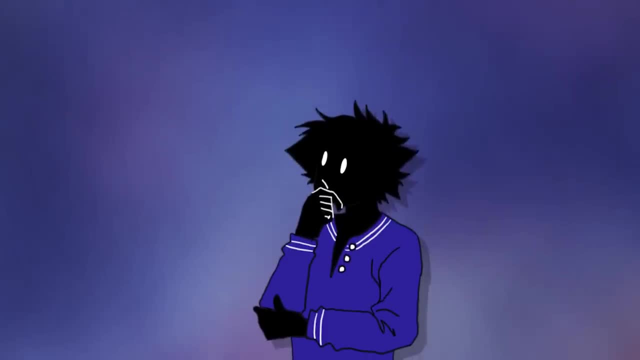 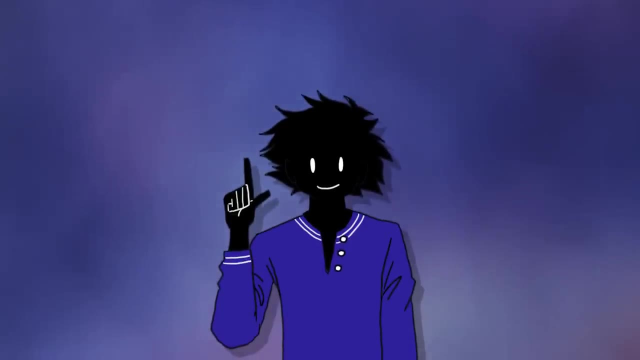 systems. It was also used to manage electronic health records. Its code tends to be very terse, which means you can take most of its word commands and abbreviate them into simple short letters. LOGO, An educational programming language made in the 60s which makes use of what is known. 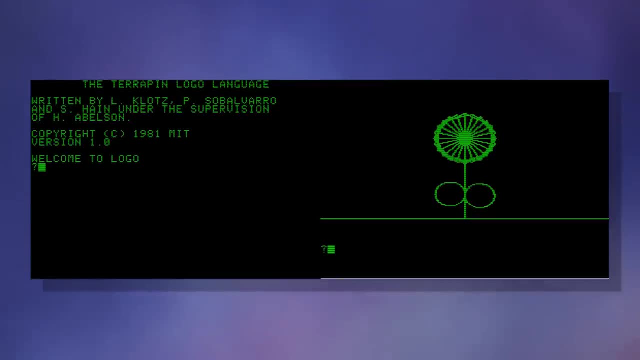 as a turtle graphic, not an actual turtle. It's the name of the cursor used to draw geometric shapes, as determined by the code PASCAL, A programming language that was very popular in the 70s. Even being the default language, it's still used today. 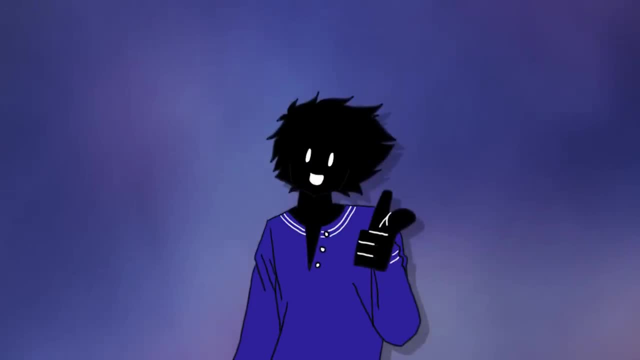 TURTLE GRAPHIC. TURTLE GRAPHIC was the default language for many computers back in the day. It was one of the first programming languages to be used by an IDE, which is an integrated development environment, Basically a dedicated program to write its code. One of the most 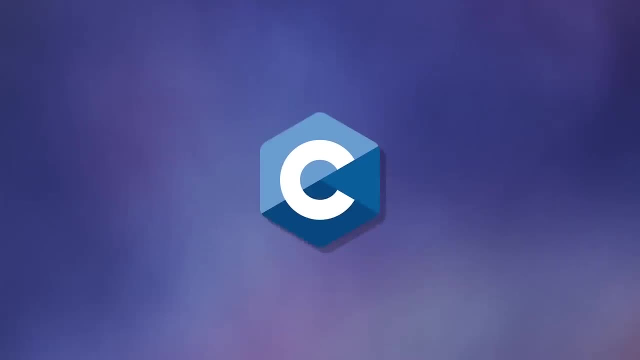 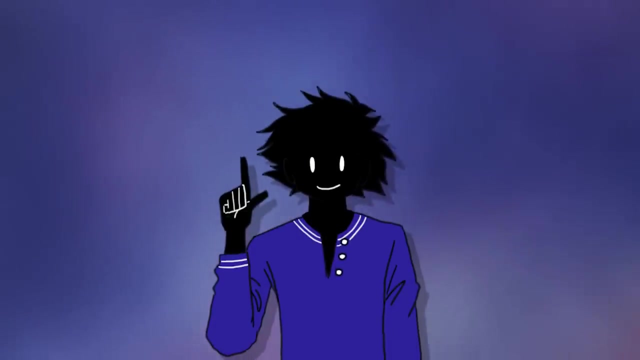 well-known programs created with Pascal was Photoshop C, A programming language created in the 70s that is one of the most popular programming languages of all time. Created at Bell Labs, it is the basis of many operating systems, such as Windows and Linux. It also inspired many programming languages that came after. 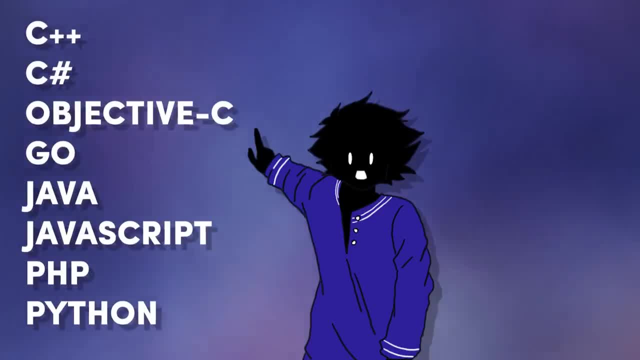 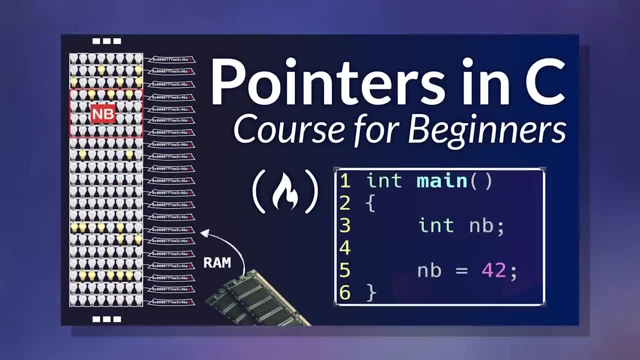 it, such as C++, C, Sharp, Objective-C, Go, Java, Javascript, Python and so on. It's known for its low-level access to the computer's memory by using code called pointers. Computer memory was much more of a finite resource in the past, so programmers had to. 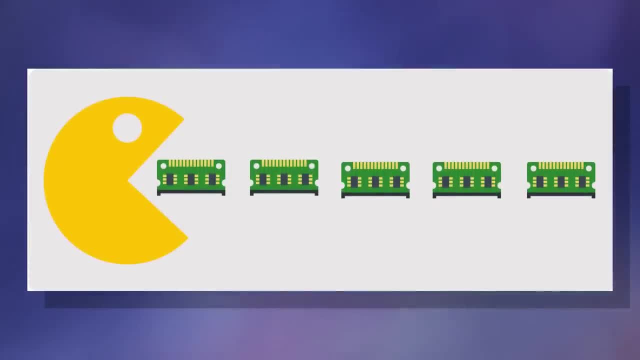 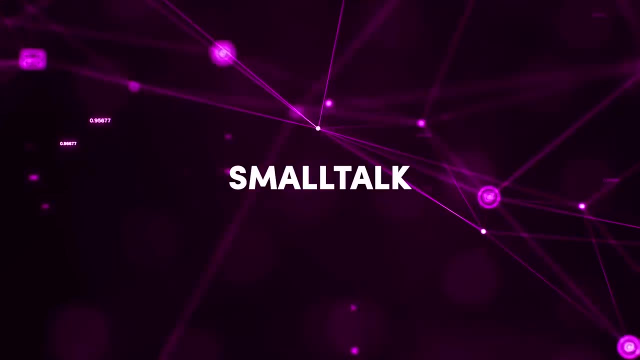 be much more careful about how they allocated it. Otherwise it'll cause problems such as memory leaks, which is basically when programs use up too much memory in your computer, causing the computer to become painfully slow. SMALLTALK, A programming language in the 70s that was known for its object-oriented programming. 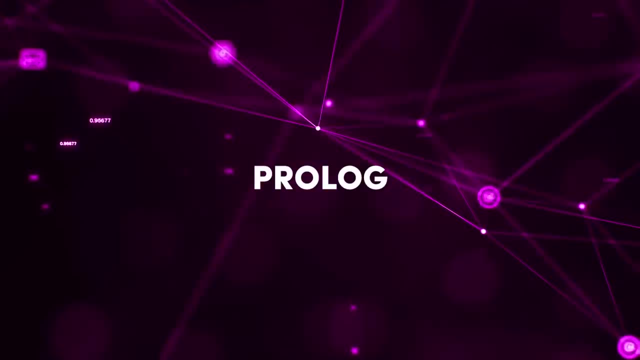 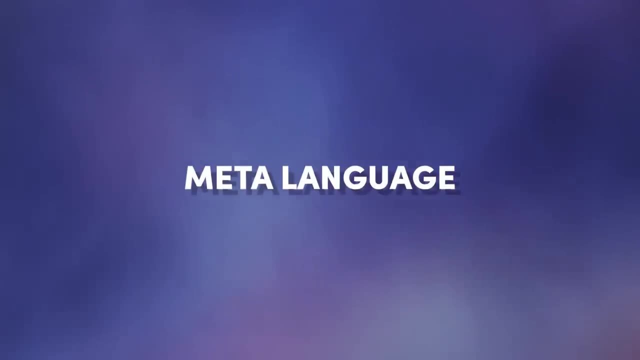 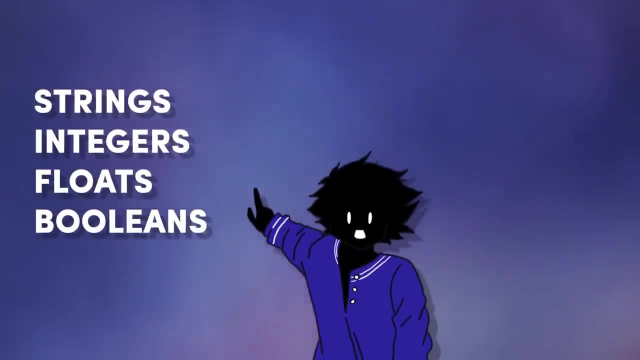 It inspired many object-oriented programming languages that came after it. Known as the first logic programming language, it is known for being modeled after formal logic in philosophy. ML, Also known as meta-language, pioneered statically-typed functional programming, which basically means giving information. certain types such as strings, integers, floats or booleans Strings. 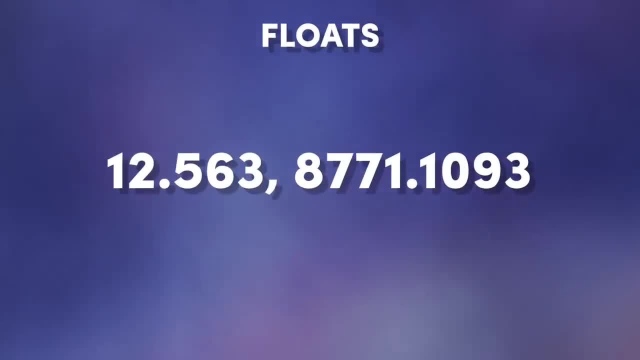 are just words and letters. integers are whole numbers, floats are real numbers, so they can be decimals, and boolean is something that can be either true or false. SQL- SQL, also known as Structured Query Language, also even called SQL, is a language used for 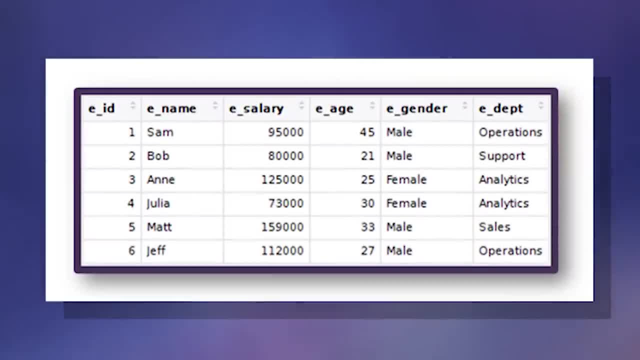 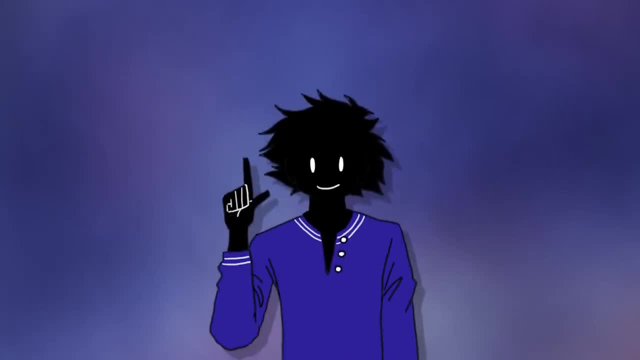 creating and managing databases. You store information in things called tables and structure them with rows and columns. The code also looks like plain English sentences. It is used by many systems, even today, to store their data, such as usernames and passwords transactions. 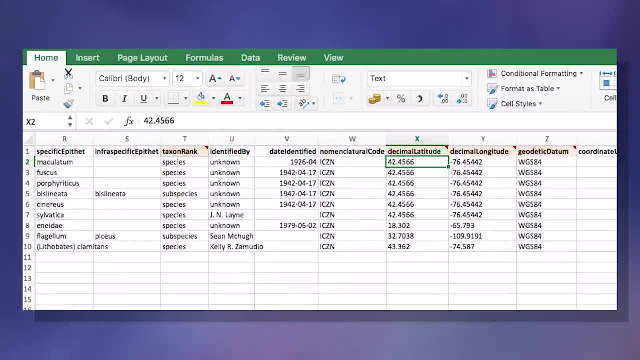 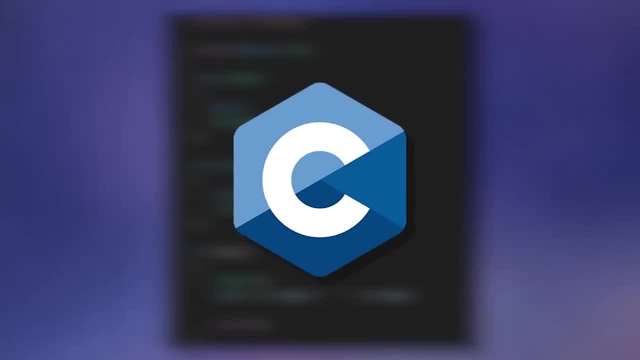 account information and, more Basically, think of it as the system of Excel spreadsheets, C++, An extension of the C programming language. The major difference is: C++ has object-oriented programming, unlike the original C, which didn't. It's also known for its steep learning. 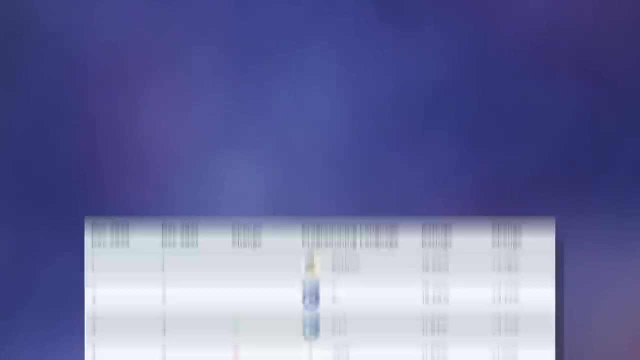 curve. C++ is one of the most important programming languages of all time, Even though it's a very complex language. it's still a very complex language. It's a very complex language and it's still in wide use today, still being the main programming language in creating. 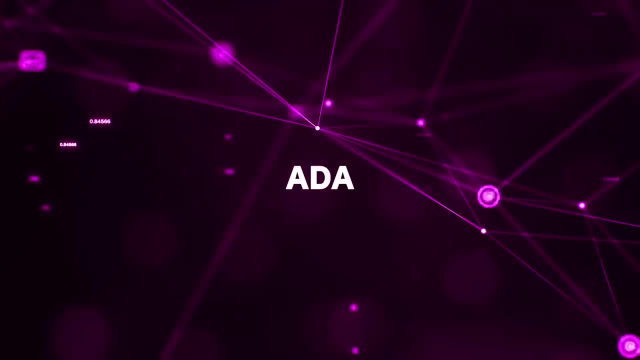 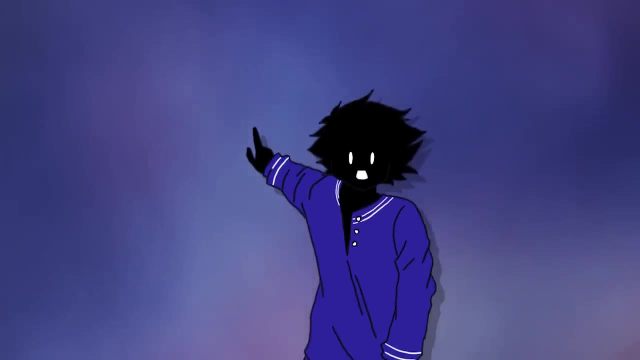 operating systems, web browsers, databases and games. Ada, A programming language made in the 1980s that is mainly used by the US Department of Defense. It is named after the credited world's first programmer, Ada Lovelace. 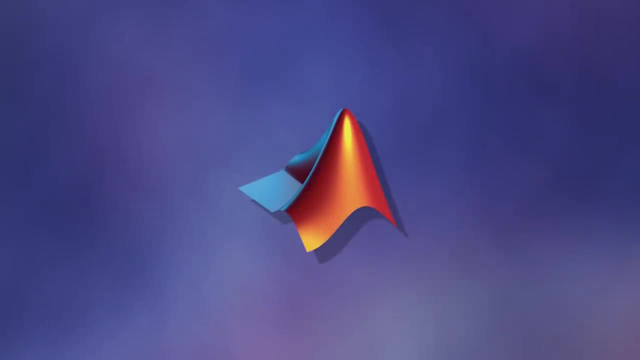 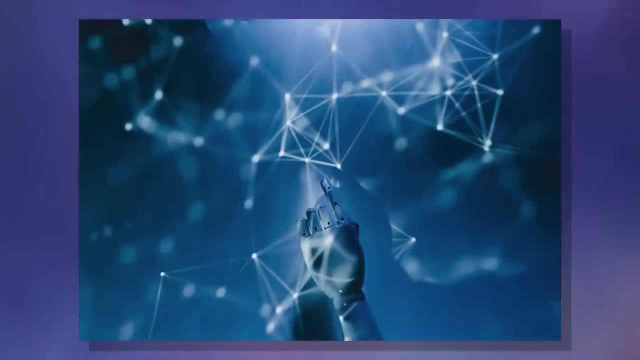 MATLAB. MATLAB or Matrix Library is a mathematics programming language used by data scientists and engineers. It's a mathematics-based programming language that can be used for statistics, robotics and artificial intelligence. It's still widely used today, mainly due to the use of computer-based programming. 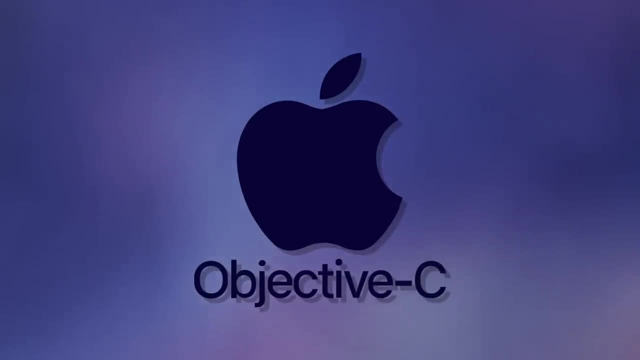 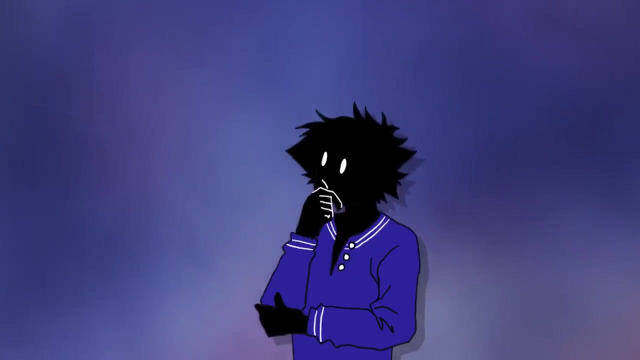 Objective C, A programming language inspired by C that was created in the 1980s, which became the main language for Apple computers, even being the main language for the early iPhones, Although its popularity has fallen over the years, mainly due to Apple replacing it by a newer. 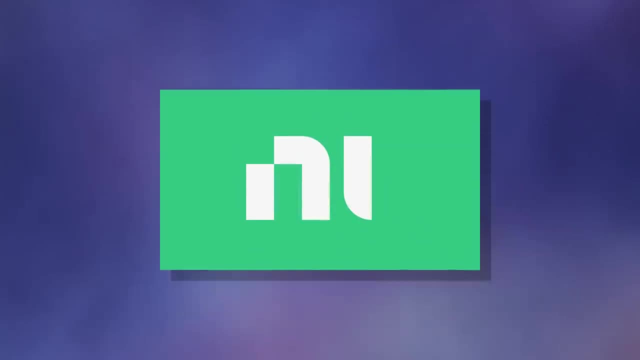 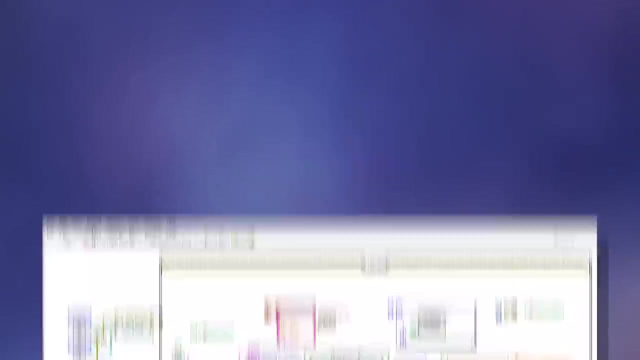 programming language called Swift in the mid-2010s LabVIEW Made by National Instruments in the 1980s. it is a programming language that doesn't really use traditional code. Instead, it's a graphical programming language where you build user interfaces and handle code using images. 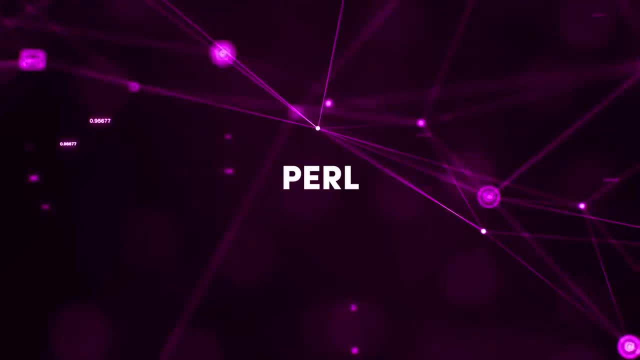 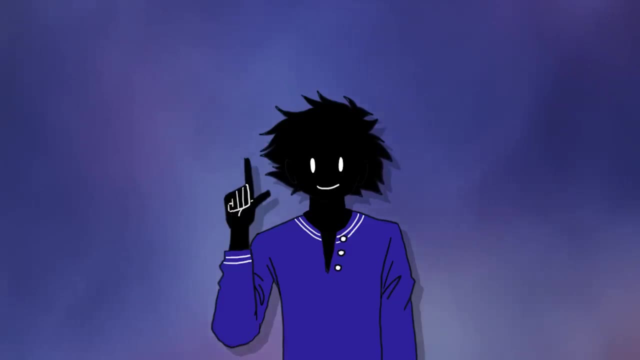 Erlang, A programming language designed for the telecom industry, Perl, A language that was designed to work very well with text. It's used for system administration, network programming, finance and more. Perl has been known as the duct tape that holds the internet together. If you've ever seen the code, it actually looks pretty wacky. 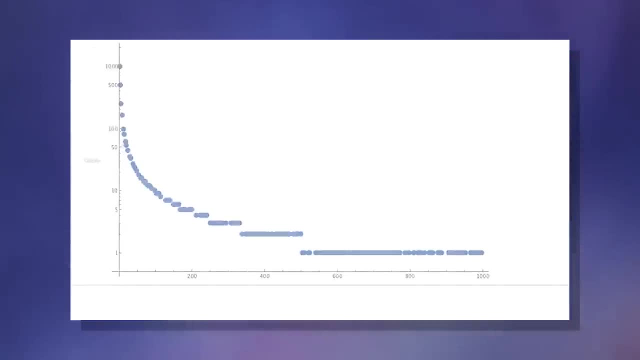 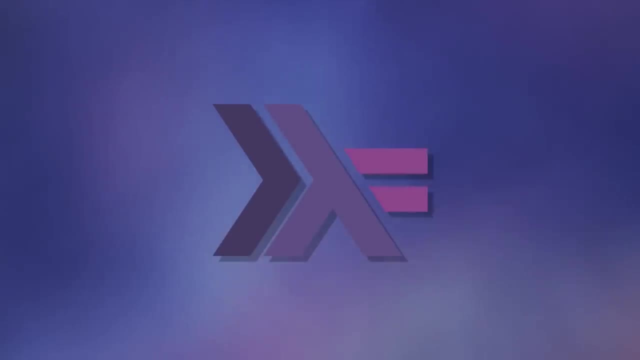 Wolfram. Created by Steven Wolfram, it's a language that can perform data visualization, image processing, mathematics and pretty much anything you can think of. It can even tell you the shortest route around Europe- Haskell. It's a functional programming language, with its unique feature of its variables being 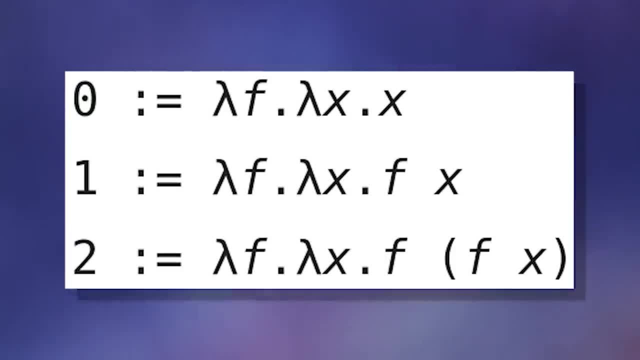 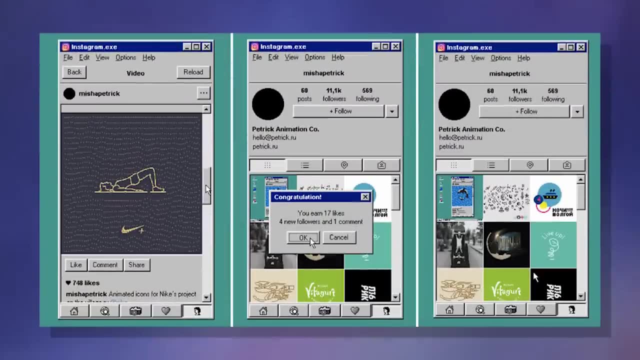 immutable, which means you can't change them. The language is based on the language that comes from lambda calculus, Visual Basic, A programming language developed by Microsoft in the early 90s. It's used to create Microsoft programs and applications by using GUIs or graphical user interfaces- Basically anything. 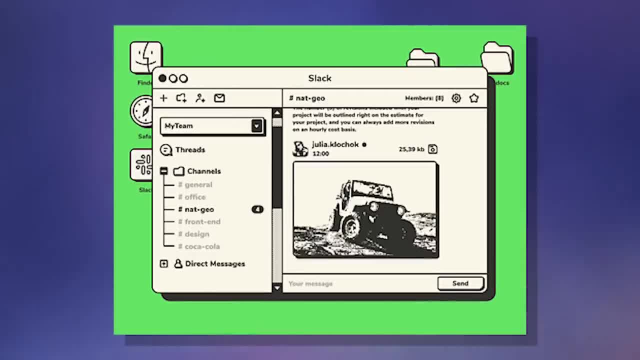 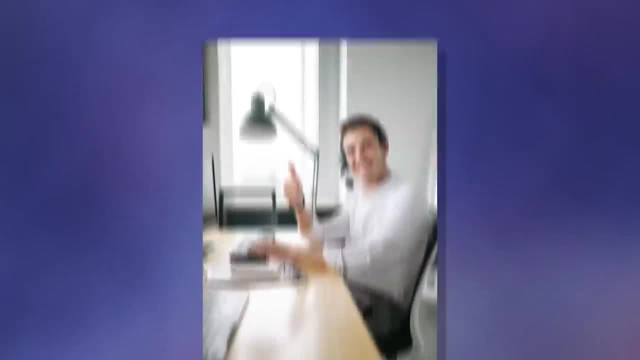 you can interact with with your mouse on the screen is part of the graphical user interface. It also has a very popular IDE of the same name, Lua, A language known for its speed and being able to be embedded into other programs. It's also known for being very easy to learn. 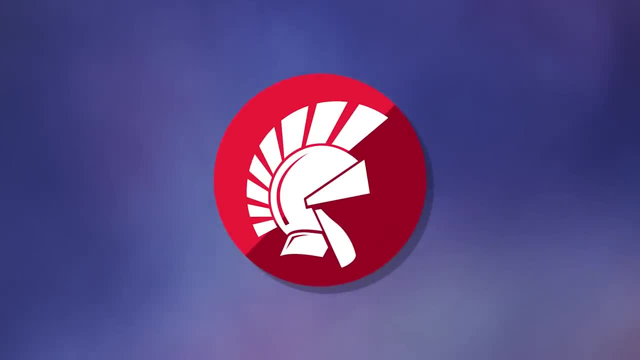 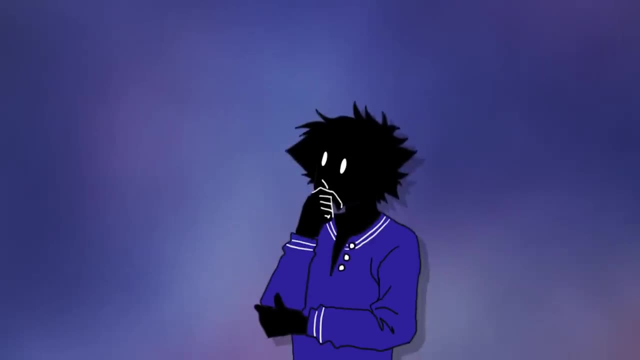 Delphi. Nothing much to say about it. It's basically Pascal, but with object-oriented programming. It even comes with its own code editor, OCaml. OCaml is a functional-based programming language, like Haskell and Erlang. Functional programming languages are good at doing math, and object-oriented programming languages are good for building. 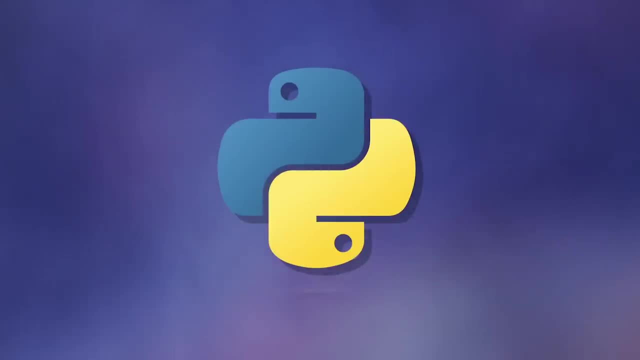 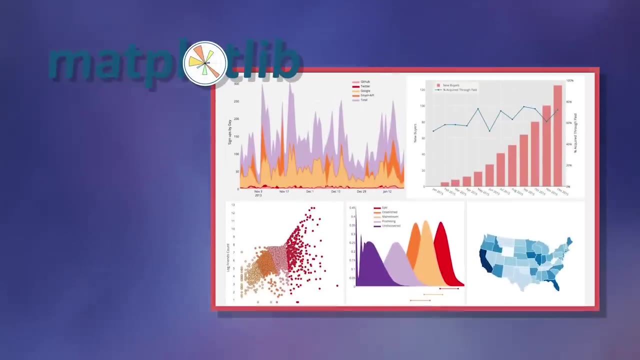 enterprise-level software Python. Python is a general-purpose programming language, and you can use it to make pretty much anything From desktop applications to websites, creating bots or API, handling servers and databases, game development, image processing, statistics and so much more that it would need its own. 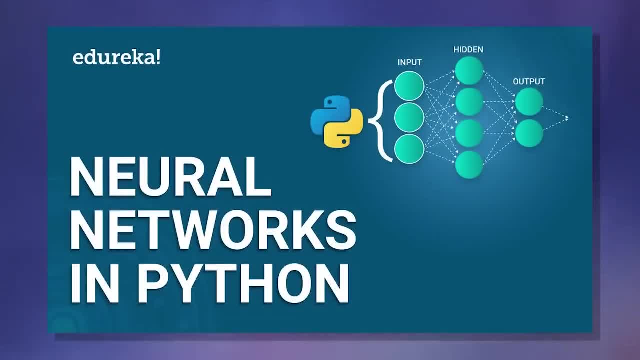 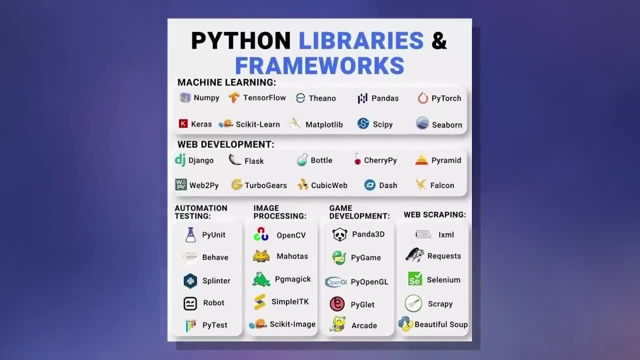 video. Python is currently one of the most popular programming languages for creating AI. It's also one of the most popular programming languages in general. In fact, most beginner programmers start with Python as their first programming language, not only for its vast utility, but 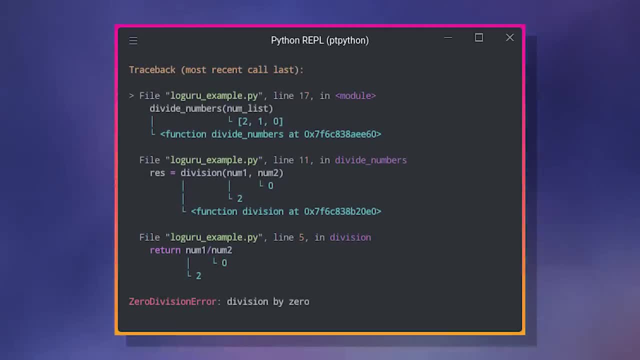 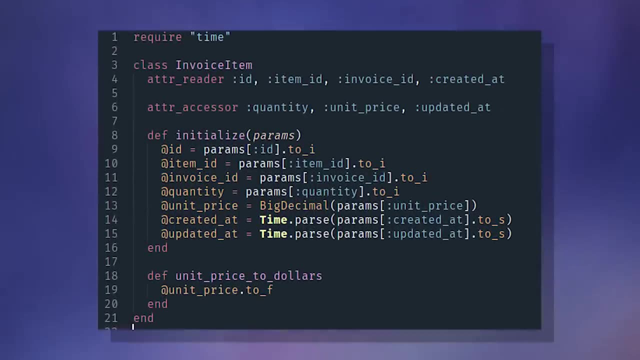 also how easy it is to learn. One of its only drawbacks is that it tends to be pretty slow compared to other programming languages like C++, Ruby. Ruby is a language very similar to Python. Even the code looks similar. Ruby is easy to learn and the code is also very readable. One of the most popular uses of Ruby is to: 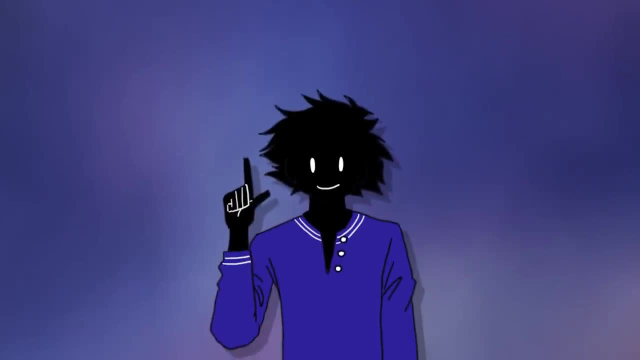 combine it with a framework called On Rails to create websites, adopting the full name Ruby On Rails. Ruby On Rails is currently being used as an online website, but it's still a very popular programming language in general. It's also one of the most popular programming. 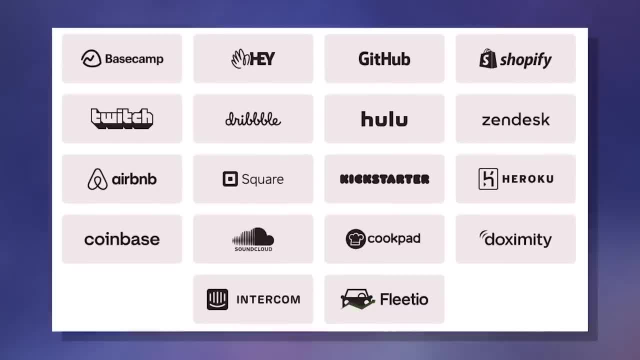 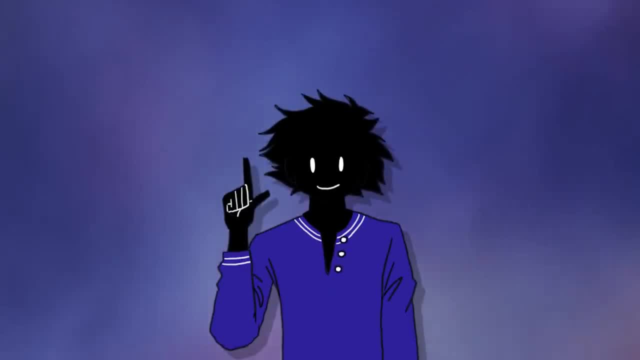 currently the backbones to many websites we know currently, such as hulu, airbnb, coinbase, shopify, twitch, soundcloud and many more. a lot of its popularity was its ability to be able to create full stack websites. full stack is the combination of the front end and the back end development of a 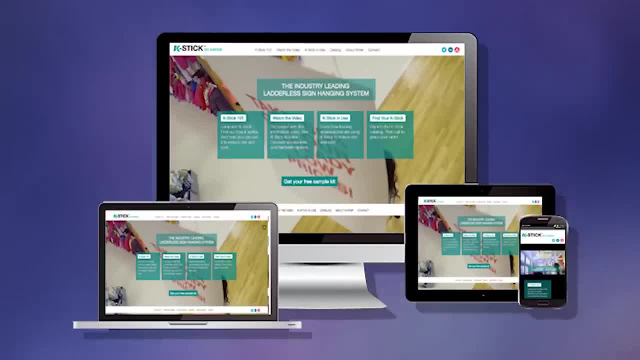 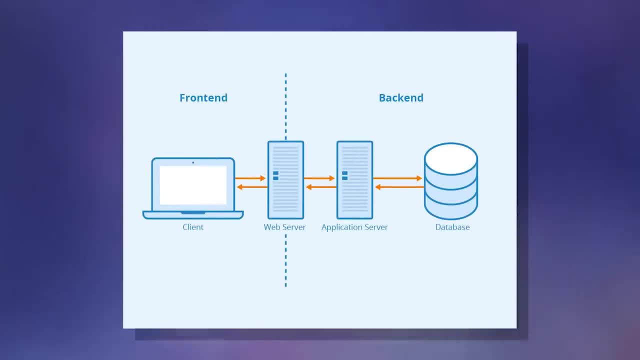 website. a website's front end is basically everything you can see with your eyes, basically the entire interface. the text, the images, the buttons and the videos are all part of the front end. the back end is the non-visual part of the website, which is mainly the servers and 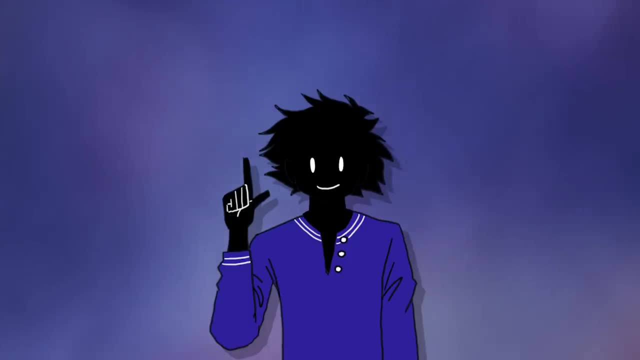 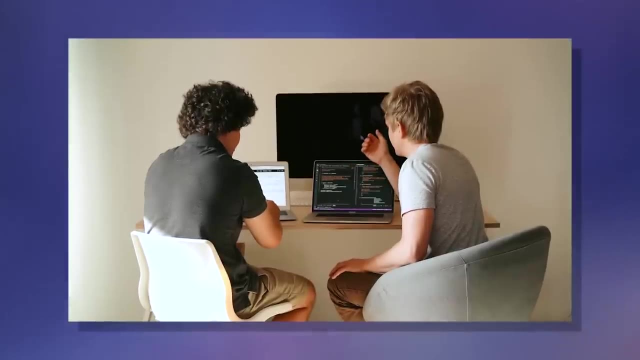 databases, account information, authentication and data storage is what's part of the back end java. remember the thing some programs ask you to install on your computer. yeah, that's an actual programming language. it gained popularity immediately after it's released and it's still popular today. a big advantage that java has is that it allows you to create programs that are 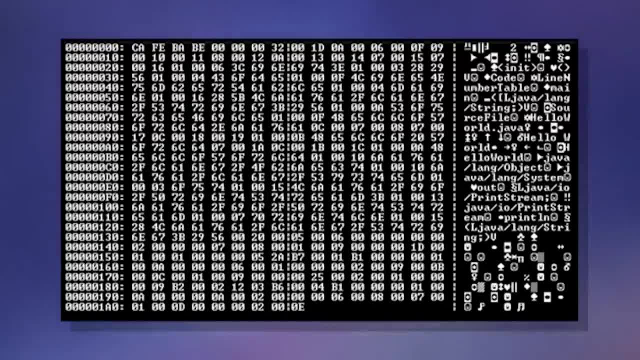 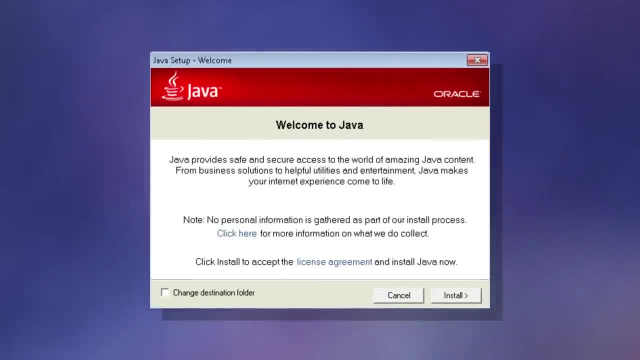 very platform, independent. that's because java can be compiled into bytecode which can be understood by many operating systems. all your computer would need is a java runtime environment to do this, which is what you're installing every time your computer asks you to install java. java can be used. 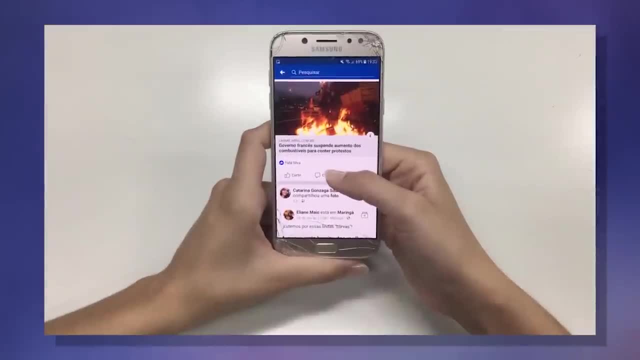 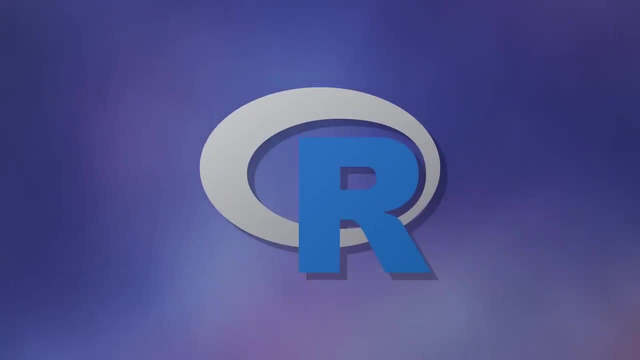 to create many things like video games such as minecraft, or mobile apps on android. a meme amongst beginner programmers is that java's code tends to be pretty verbose. are a programming language in which its main purpose is statistics. it's a widely popular programming language used to organize data. 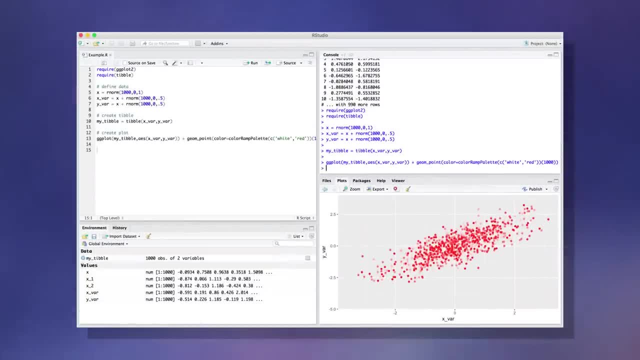 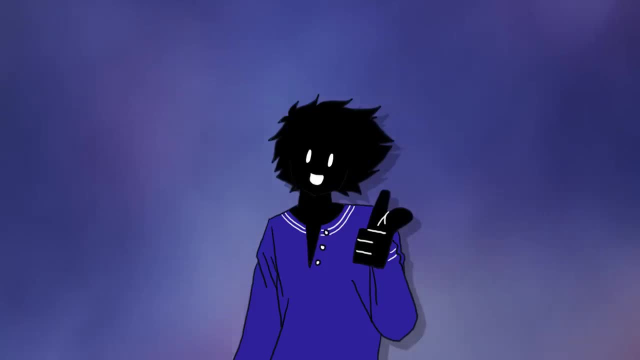 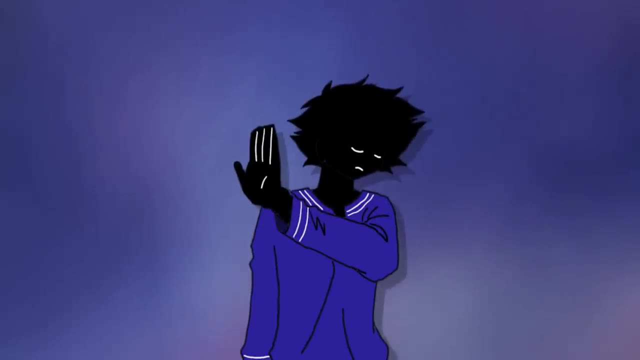 and data visualization. it's very useful for researchers conducting epidemiological studies. if you're a researcher studying in fields such as economics, psychology, biology, medicine, etc. learning how to code in either python or r is a very useful skill. javascript- javascript is not the same as java. in fact, it has nothing to do with java. javascript is a programming language that is mainly only used. 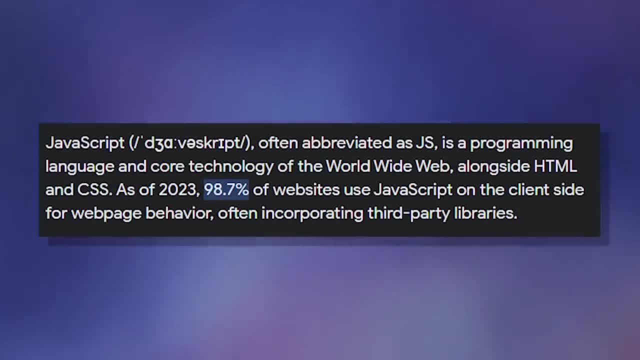 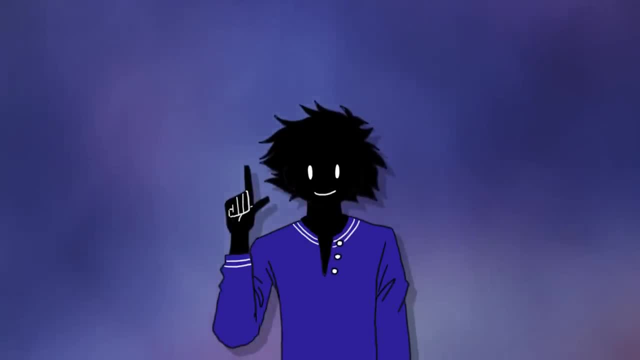 in web browsers. in fact, 98 of the internet uses javascript. javascript is responsible for the main functional aspect of the website. it's based on the ecma script standard and is often used in conjunction with html and css, but sometimes you can create websites with just pure javascript. 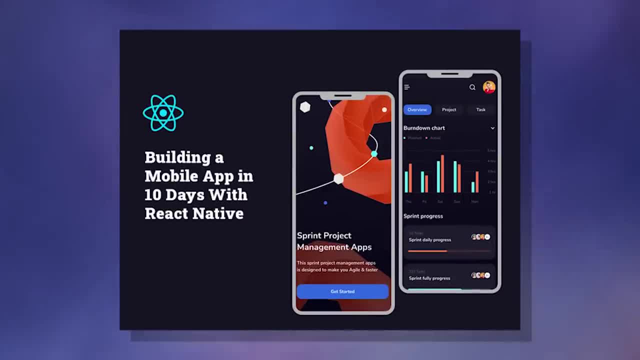 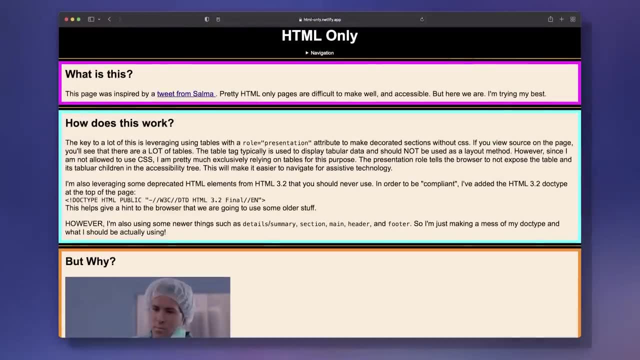 using frameworks such as react and with react mobile, you can create mobile apps. html and css. html and css are both scripting languages to create websites. html deals with the pure code of content and structure of the website. it uses code called html tags in order to build the content on. 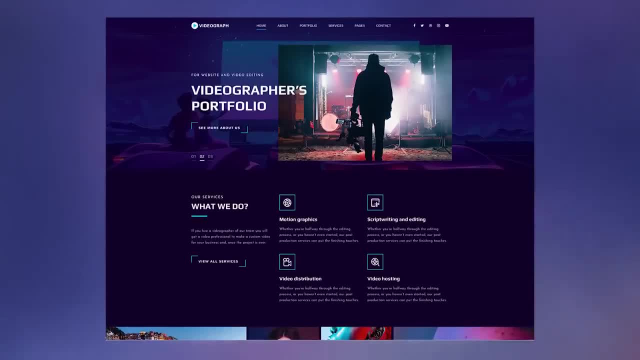 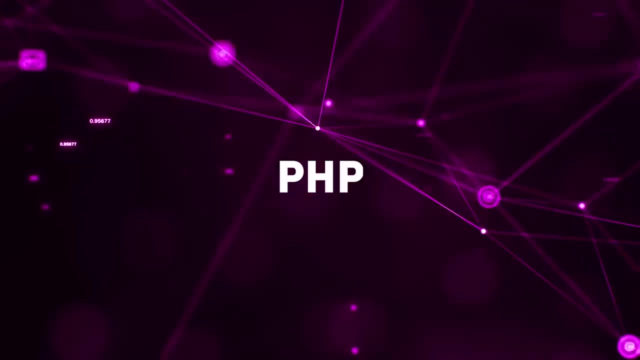 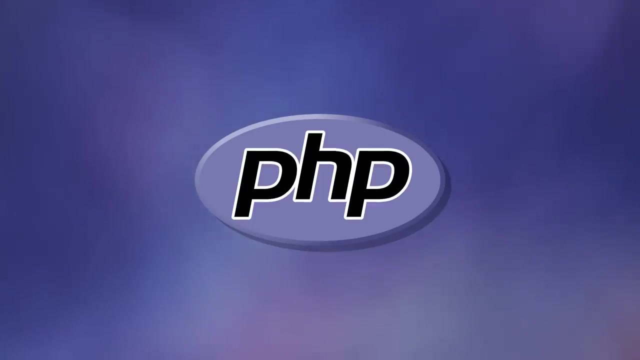 the webpage. css is used for the design or aesthetic look of the website. it deals with the arrangement of content, colors, borders, gradients, opacities, and can even perform animations. php- php, aka personal home page, but sometimes also called hypertext preprocessor, is a programming language mainly used. 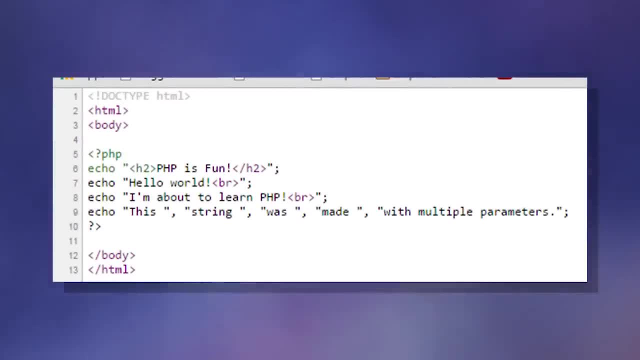 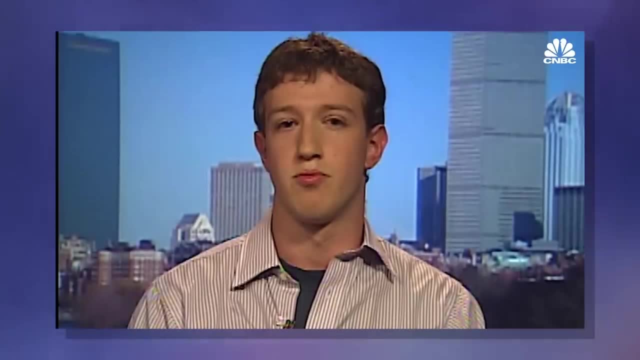 on web servers, you can actually embed php directly into html. php, although waning in popularity, is many major websites today. it was the language mark zoggerford first built facebook in action script, a language based on javascript in which its main purpose was its use in flash. have you ever 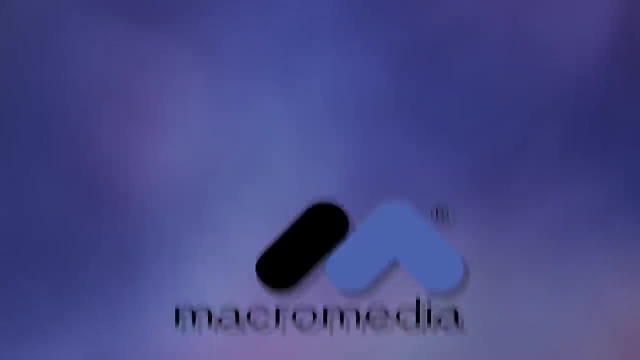 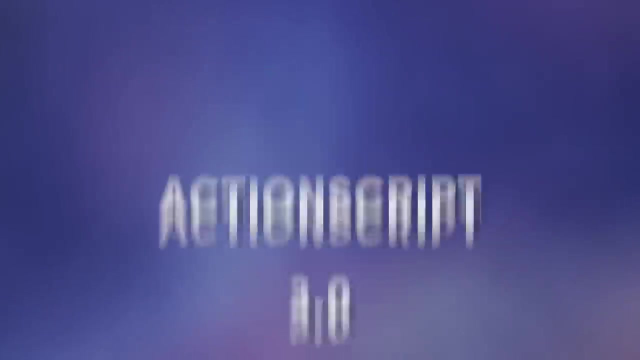 played a flash game back in the day that was most likely made using action script. it was first created by macromedia, which released action script 1 and version 2.0, but when macromedia was later bought out by adobe, adobe released action script 3.0, even though, as of 2020, adobe flash has died. 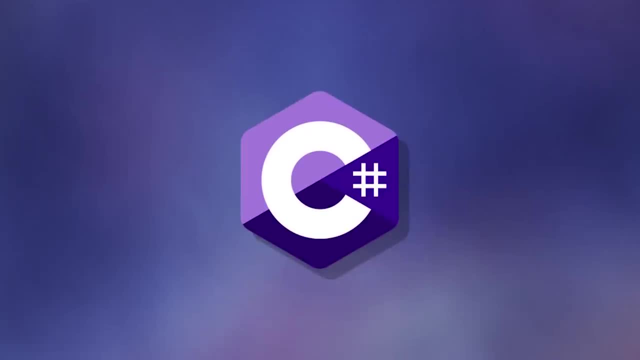 out. you can still use action script with adobe. animate. c sharp, a programming language made in the early 2010s. it was influenced by c plus plus and java. c sharp's most common uses are being used in web servers with thenet framework, and video game development with the unity engine scala scala. 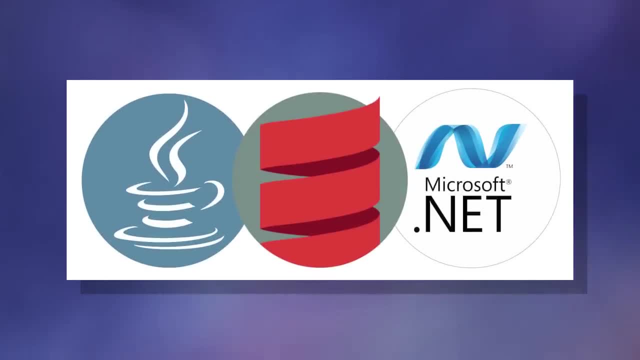 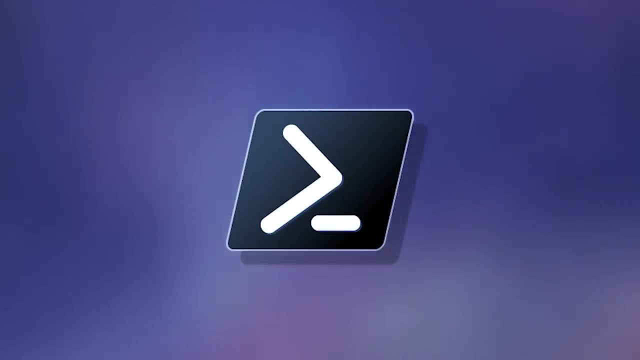 was made as an alternative to java. it also uses many of java's same technologies, such as the java virtual machine, but unlike java it has many features of functional programming powershell- basically the windows command line on steroids. come with its own scripting language, f sharp. f sharp is the sister language to c sharp, with the difference of it being able to support functional 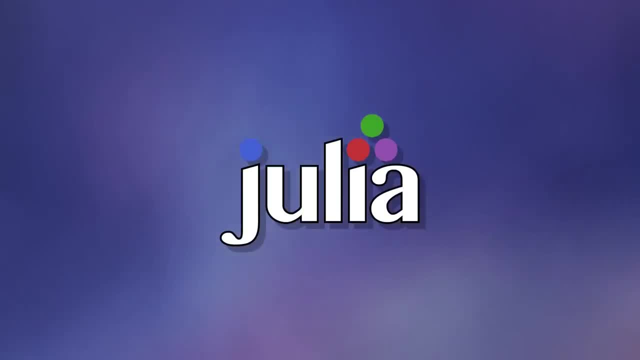 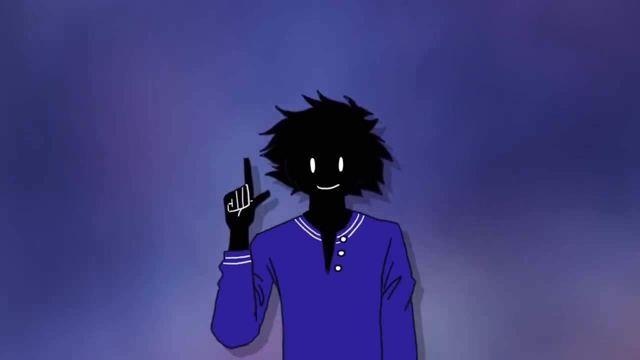 programming julia, a programming language made in the early 2010s and is used in a variety of games in order to perform high level computations, data analysis and visualization, and mathematics. its main advantage is that it's much faster than other programming languages that do this. the code is a. 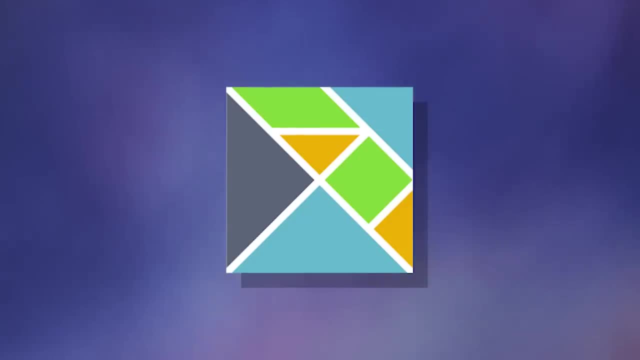 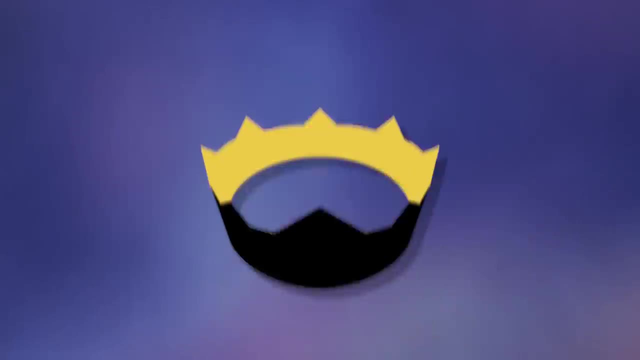 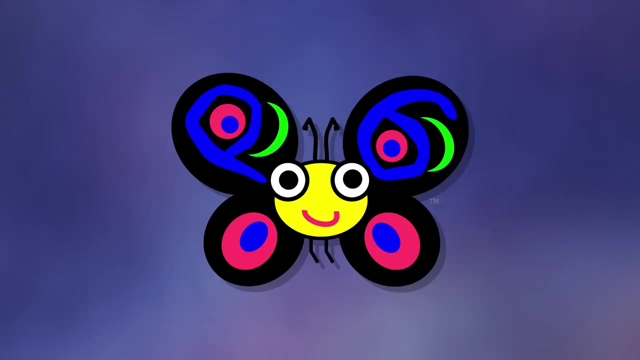 lot easier to read and it's much easier to learn home, a programming language designed to create graphical user interfaces for websites. it can be compiled into javascript, nim, a programming language with the simplicity of python, combined with the memory allocation of c. plus plus roku, nothing much to say, it's basically pearl. but version 6, although it has a pretty wacky logo, scratch a programming. 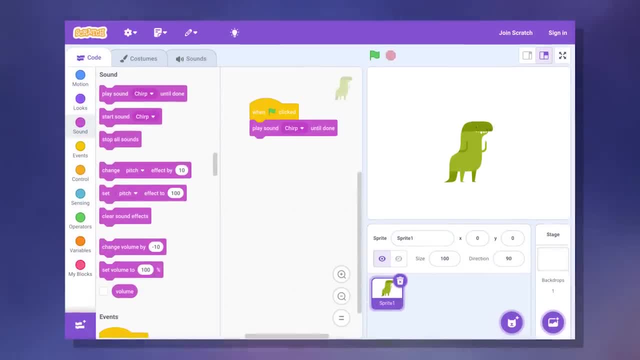 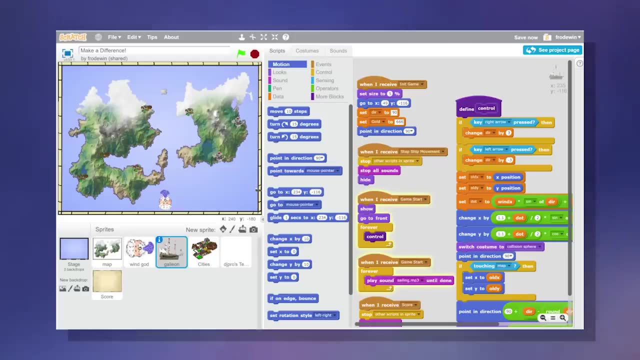 it that is completely visual and block based. no, seriously, the code fits together like lego blocks. it was made with the purpose for teaching children how to code. despite its simplicity, you can make pretty complex things with it. go. formerly known as golang, was created at google to be a modern 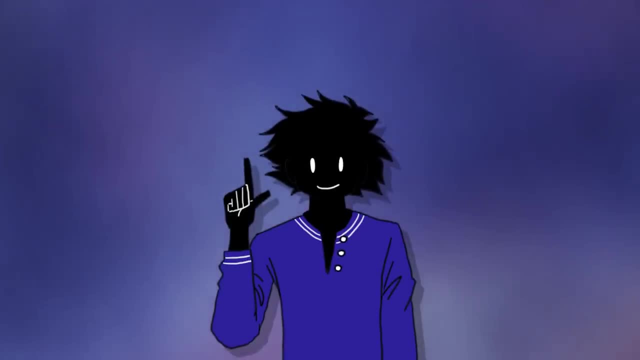 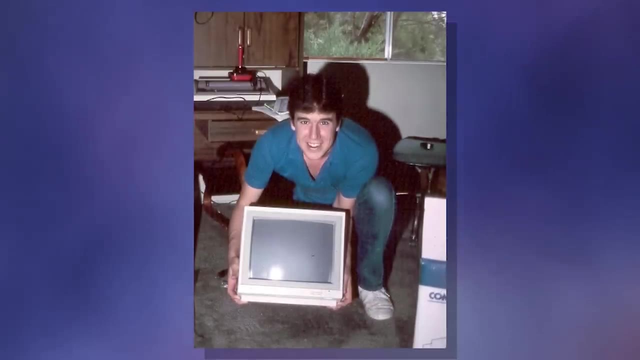 version of c. the code can be similar to python, but it's much faster due to its compiling method. it's mainly used in servers with frameworks like docker holy c, a programming language created by terry a davis in 2005.. made with assembly, it was used to create an operating system called temple. 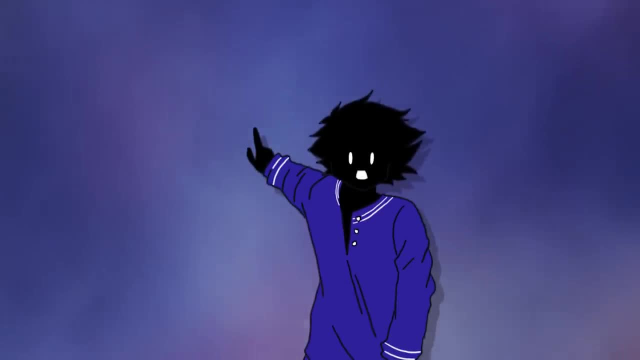 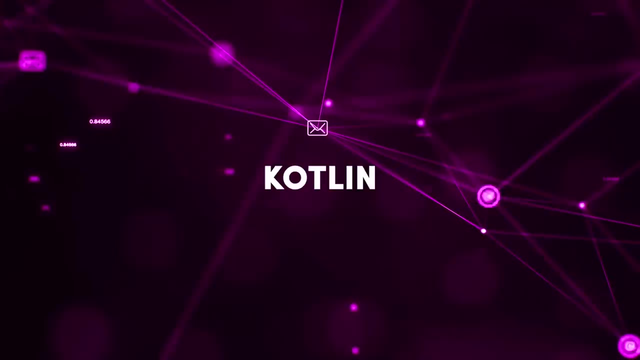 and it was also used to create a computer system inspired by a revelation from god. the main interest in this programming language is due to the backstory of the developer, although being a talented programmer, suffered from and ultimately succumbed from his battle with schizophrenia. kotlin, known as the easier form of java, is a language used to create mobile apps on android os. 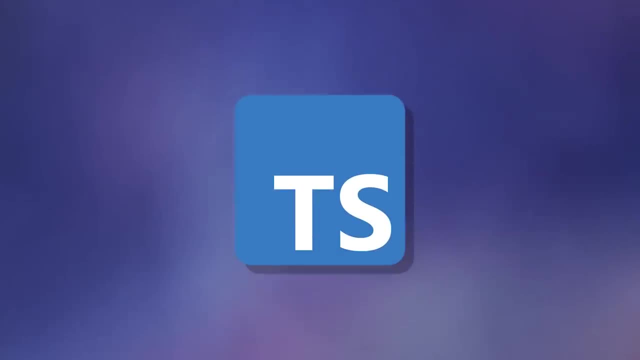 the most popular ide to code kotlin in is android studio typescript, basically javascript, but with static typing. dart, a programming language created by google that you can use to create web applications or mobile apps using the flutter framework swift developed by apple to replace objective c. it is the standard programming language to create anything in ios and it. 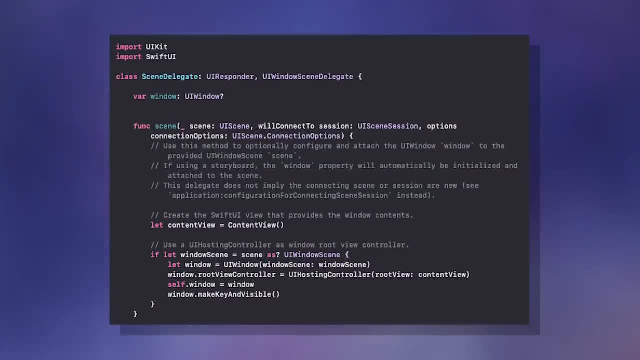 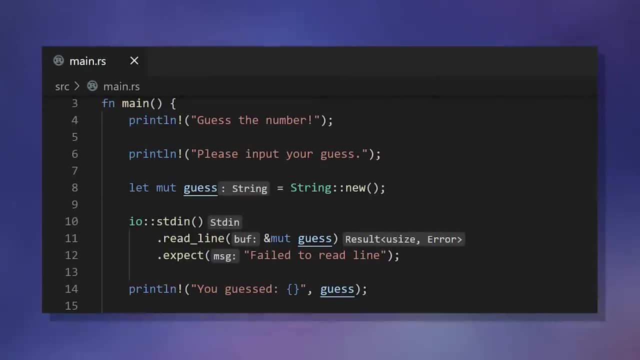 comes with its own code editor called xcode. you can only code in swift if you have an apple computer or use a virtual machine. rust okay, this is the true modern version of c and c plus plus. it's good if you want to write simple code while also handling memory issues. it's a very popular. 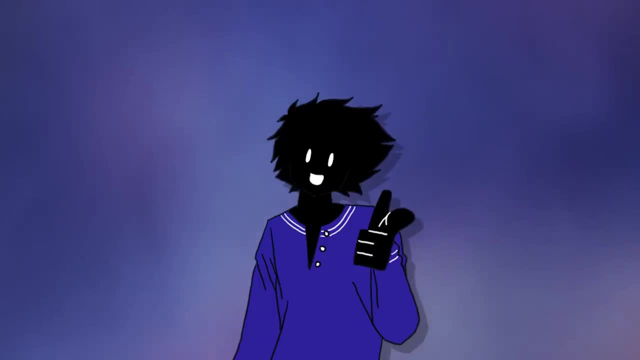 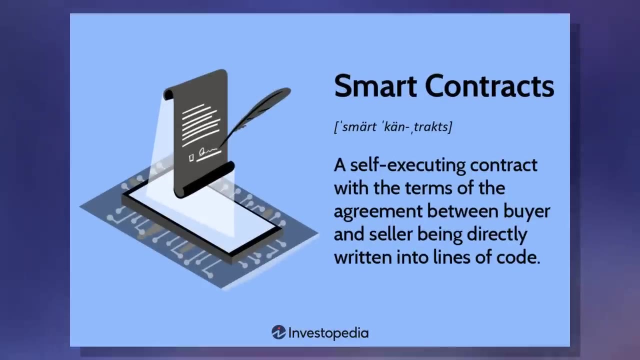 programming language, and it's used to make applications where performance is extremely important, such as game engines or operating systems. solidity, a programming language created for the ethereum network. programs created in solidity are called smart contracts. these smart tracks are later deployed to the blockchain. however, once smart contracts are deployed to the 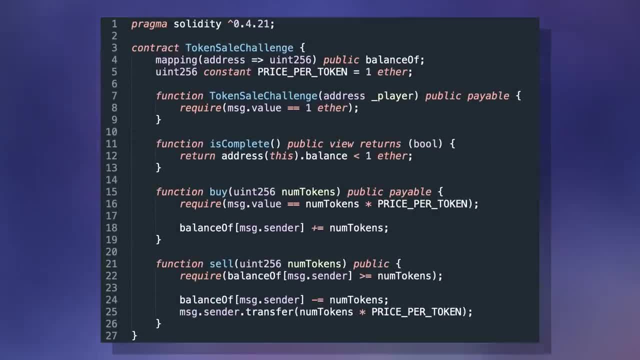 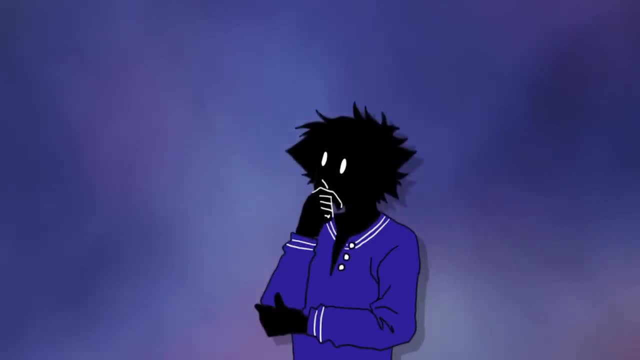 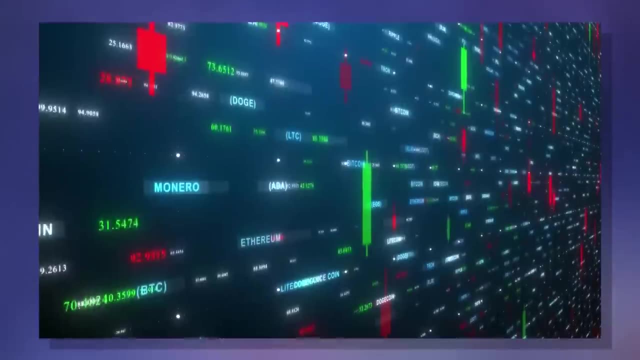 blockchain. they cannot be changed or altered again, so before a contract is deployed, usually developers test them thoroughly beforehand. this is done using testing environments such as truffle and hardhat. depending on the smart contract can cost memory and even money in the form of ethereum to work. its main uses are for creating web 3.0, decentralized apps, decentralized finance.